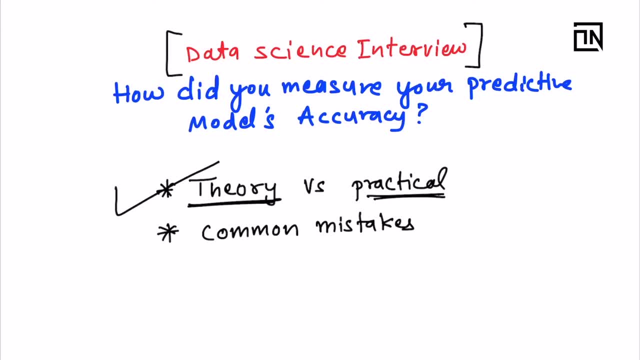 key points which you should make sure are present in your answer, And after that I'll discuss about some of the common mistakes which young data scientists in the industry make during their initial parts of the career. You should avoid these mistakes Because this may lead to the rejection of the predictive model which you have built. 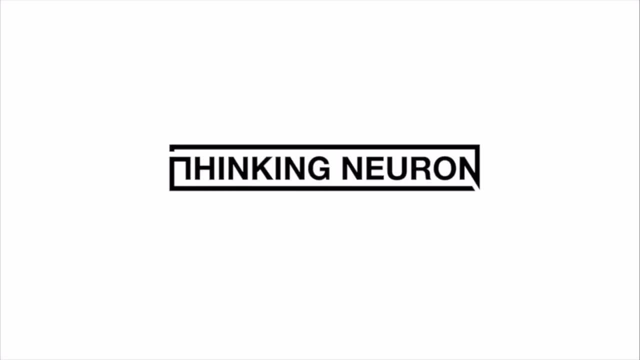 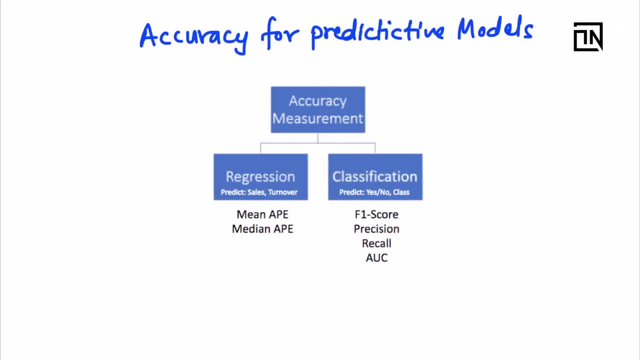 All right, so let's get started. The ideal answer for measuring the accuracy of predictive models is different for regression and different for classification. For regression, the answer is 100-MAPE. And what is MAPE? The Mean Absolute Percentage Error. So what do we mean by absolute? 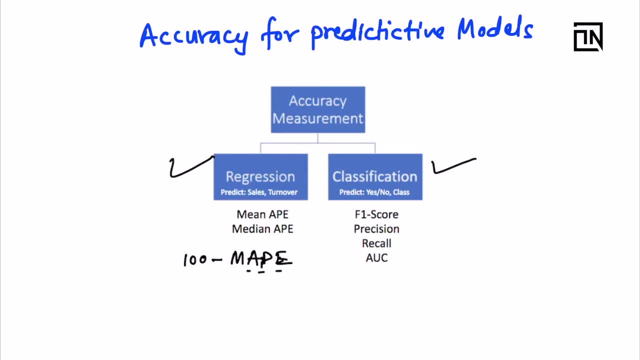 percentage error and why it represents the accuracy. I'll discuss that shortly. And along with mean, you can also utilize median for regression, because sometimes there are huge outliers, and to nullify its effect you can look at the median For classification. the one-point answer is 100-MAPE. 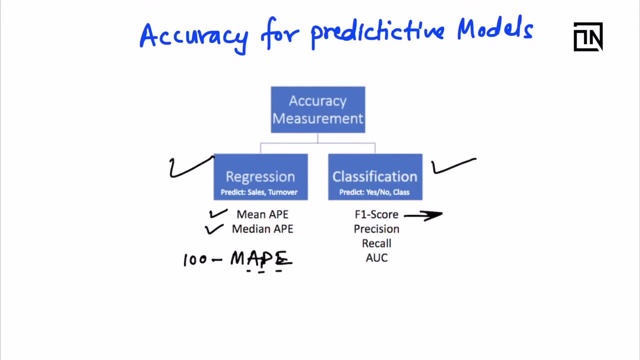 And after the decision of the algorithm, the answer, for accuracy purposes, is F1 score. So the moment you say F1 score, I will understand that, yes, you have explained this to a client, or at least you have practically implemented it, if you're answering F1 score. 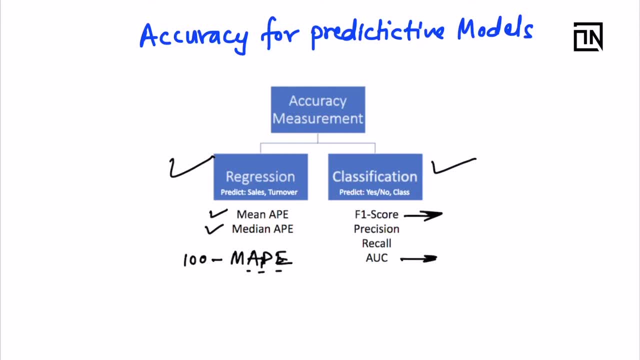 As compared to AUC, because AUC is good for binary cases. the moment you have multi-class classification, like the classes, like what is the priority of the incoming ticket. So P1 or P2 or P3, you have to classify against these three values. 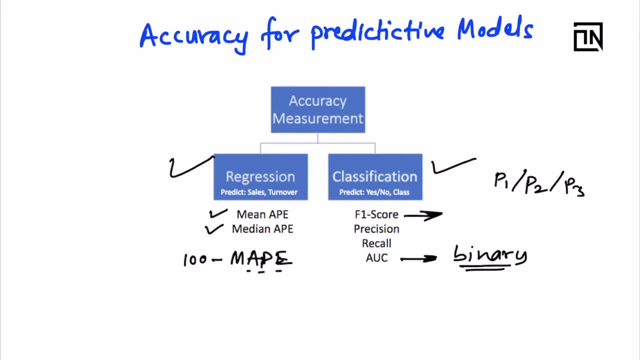 So in these scenarios the AUC can be calculated, but some extra one versus all calculation needs to be done by converting each of these levels into each of these values into one hot encoded format. So F1 score is the preferred metric. So, to sum up, the accuracy measurement for regression is done using 100-MAPE, while you 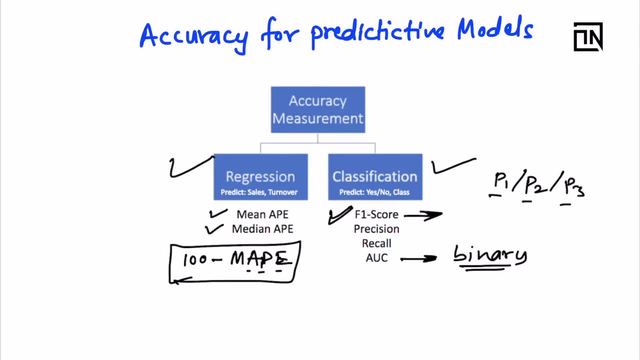 are explaining it to your client, and for classification it is done using F1 score. This is the one point classification metric. Now, F1 score is based on precision and recall. So how it is calculated and computed we will take a look shortly. A common mistake in this is when people are answering and they have learned just theory. 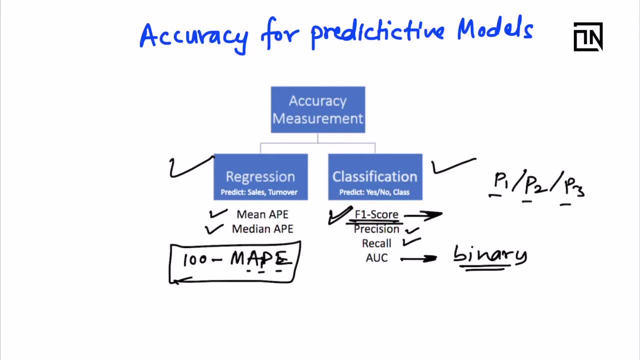 out of the jumble. They jumble up, and one common mistake people do is like when they have memorized stuff. when I ask them about their regression model, they'll say: precision, recall. I'll immediately reject that person because they have just memorized everything. 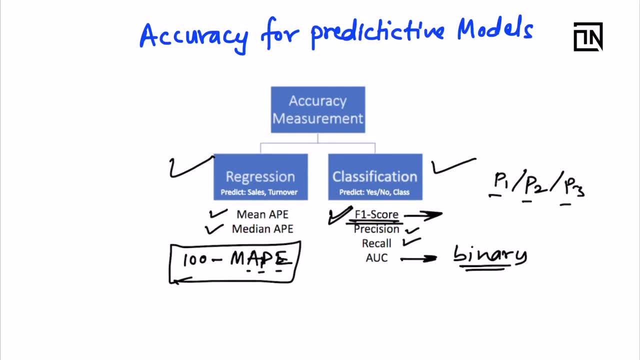 If you have really worked in the industry, if you have really implemented, then you will never mistake F1 score for regression use cases or absolute percentage error for classification use cases, Because you know these cannot be computed for the other use case, like you cannot compute APE in classification use case or you cannot compute F1 score or precision recall in regression. 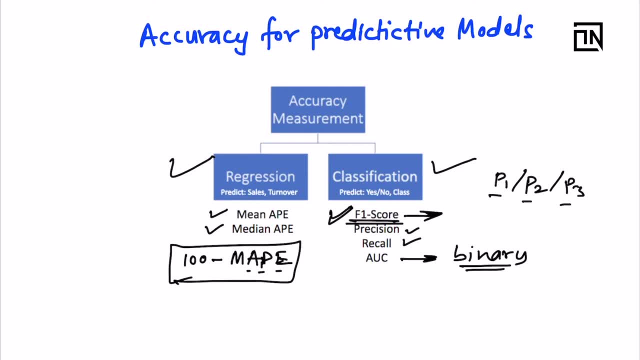 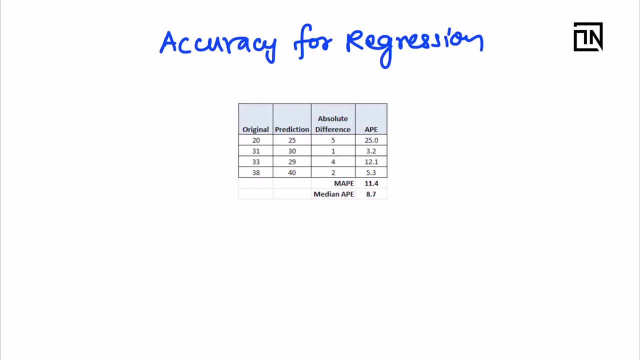 use cases. So make sure you answer appropriately. Now let's understand these in a little bit more depth. When you are calculating the accuracy for regression, you know that the regression model is producing a continuous number. So whenever you are predicting a continuous number, 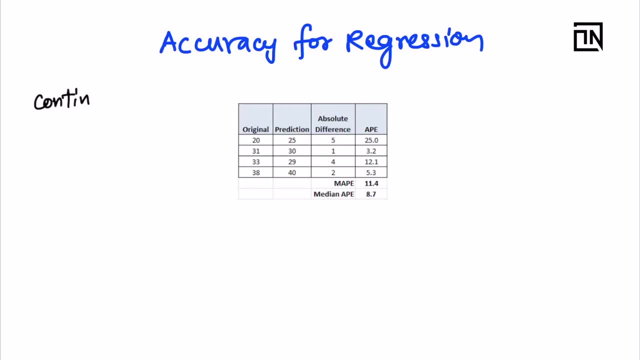 You are doing regression, So continuous number, like what? So if you are predicting the sales of an organization, or let's say you are predicting how many number of passengers will come, If you are predicting the demand of any product, like, Let's say, 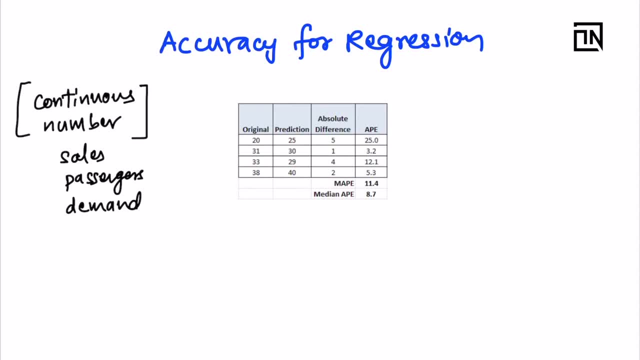 Let's say, Let's say, Dove soap. So how many units of Dove soap will be sold in the upcoming month? So you are predicting a continuous number which can vary between some range. So I'm just assuming that you are well aware of what is a regression modeling technique. 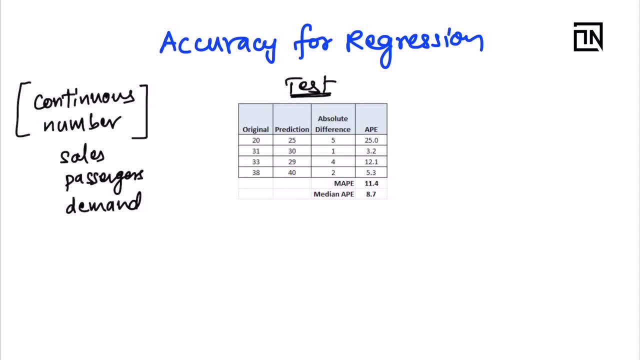 So the accuracy is computed on test data and the test data can be generated either using random sampling Or K fold cross validation, whatever the technique is, So whichever is generated. So, basically, on the test data set, on the test portion, what do you do? 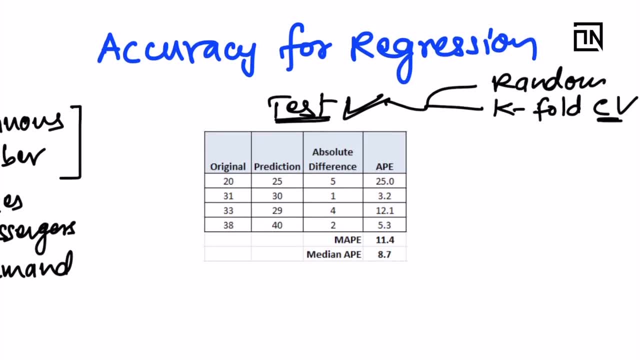 You have some original values and you have certain predictions. Like let's take, take this example: 20 is the original value and 25 is the prediction. Now what is the difference between this? So, if you calculate the mathematical Percentage difference between, 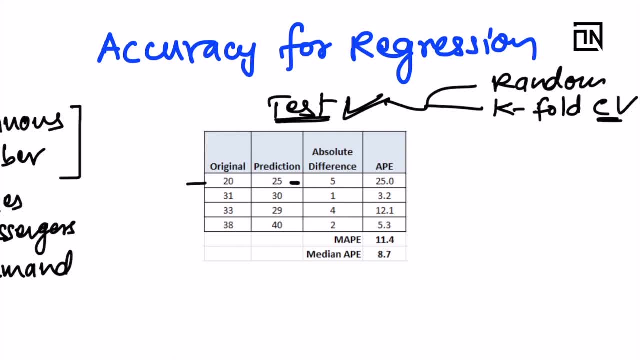 Let's say difference between 20 and 25. how will you calculate it? so the equation would be like 20 minus 25 divided by 20. so we can generalize this and put it in form of formula: original minus prediction divided by original. so this: this basically gives me the percentage difference. 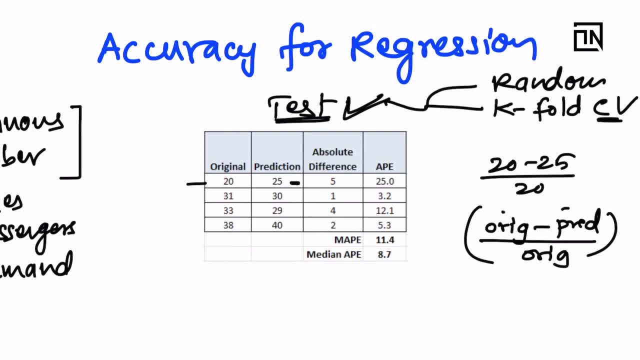 between 20 and 25, or let's say, the original and prediction. so here, as you can see, i have computed it already, so it is 25. so 25 is the error which i am making. so this is absolute percentage error, because i am taking an absolute of the numerator okay, and then multiplying it, the whole thing by 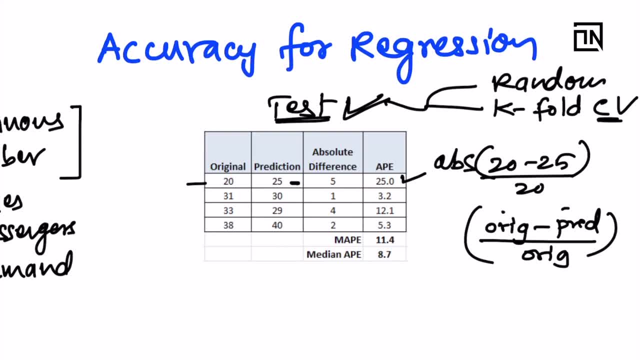 100. so when i say the original was 20 and i'm predicting it as 25, i am committing a 25 error when the original is 31 and prediction is 30. how much error i'm coming committing? how far away 30 is from 30. 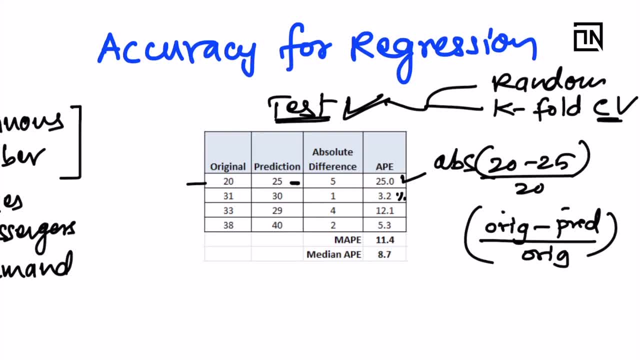 31, so 3.2 percent. similarly, 33 versus 29, it's 12.1 percent. so what i am recording here at every prediction how much error my model is making all right, and if you take the average of these errors, what you get is known as mape. and to calculate the accuracy you are doing 100 minus mape. why you are. 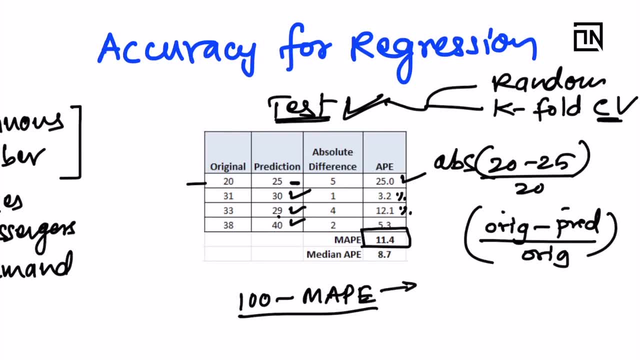 doing this because you are doing 100 minus mape and you are doing 100 minus mape and you are doing 100 minus mape. mape is the amount of error your model is making. so if you subtract that from 100, you get how accurate your model is. sometimes this mape may exceed 100 because of certain outliers. let's say: 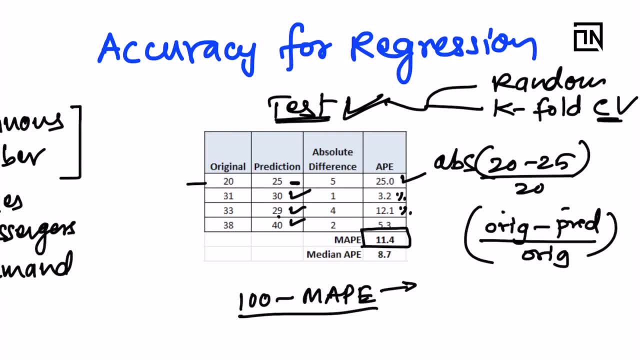 the original value was 1 and the prediction value was 200, so so it will be a huge outlier in percentage. so in such cases the mape 100 minus mape will give you negative results and for these we look at the median value. okay, when there are outliers in your test data set, all right. so you 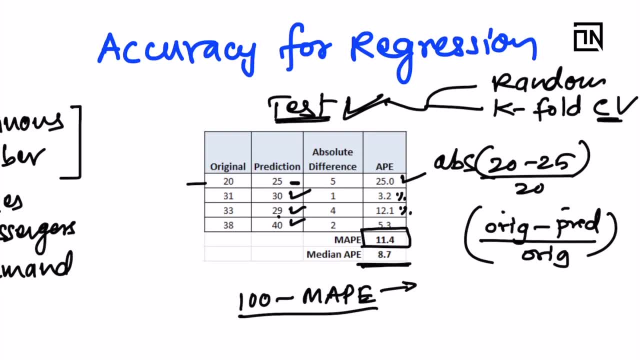 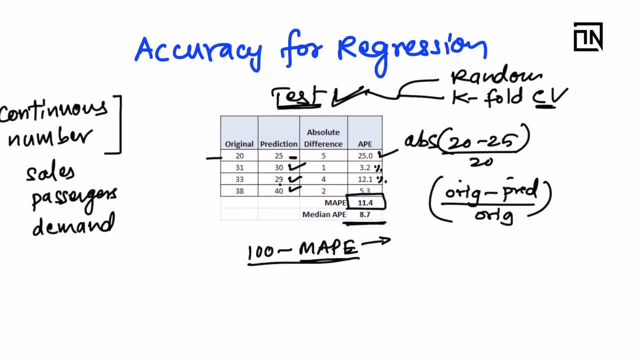 can look at this also. so 100 minus median ape will also give you an idea, all right. so so on an average, we calculate why, uh like how much error my model is making, and 100 minus that will give me the accuracy. so this is the accuracy. now other metrics which people use. 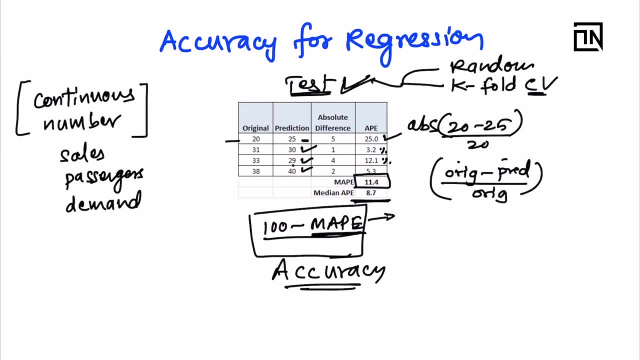 for evaluating their predictive models for regression is rmse or mse or mae mean absolute error, mean squared error, root mean squared error etc. but these cannot be explained easily to the client. the 100 minus mape metric can be explained to the client easily, that hey. 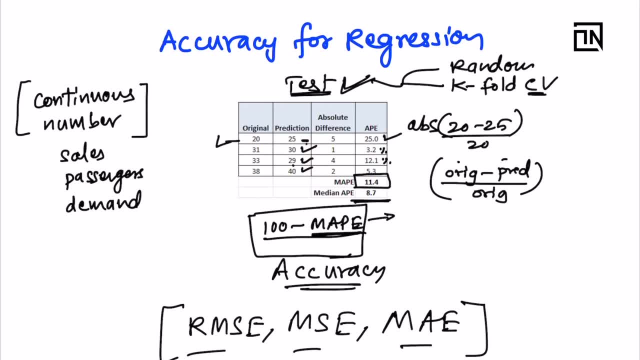 look, look, this is the original number and this is the prediction, and this is the prediction, and this is the error, and this is the error, and this is the error. and i'm just comparing how far away my prediction is from your original value. okay, so this way the client understands it easily. but if you try to give some rmse number or mse, 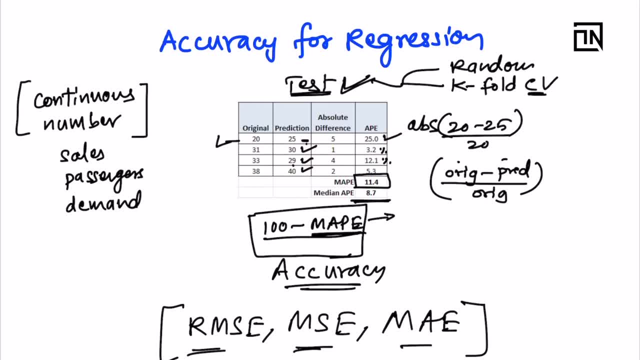 number that hey, my model is having this much mse number and it is the lowest. so that lowest number does not really make sense to the client because it's a relative thing. you can use these metrics to evaluate your hyper parameters. so when you are training, let's say 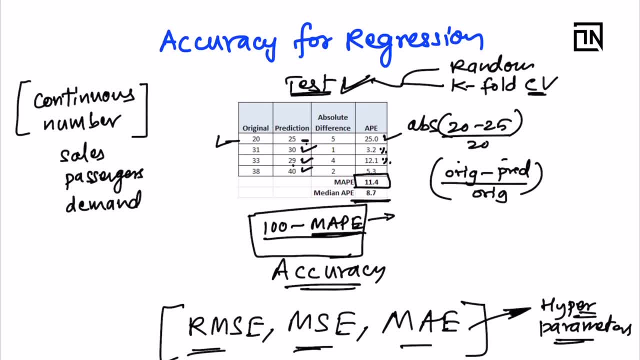 a decision tree so you can evaluate what max depth is working, what criteria is working, how many number of leaf node values are working, etc. etc. so the hyper parameters can be tuned using these metrics. but when you are deploy, when you have done tuning the model, when you are deploying, 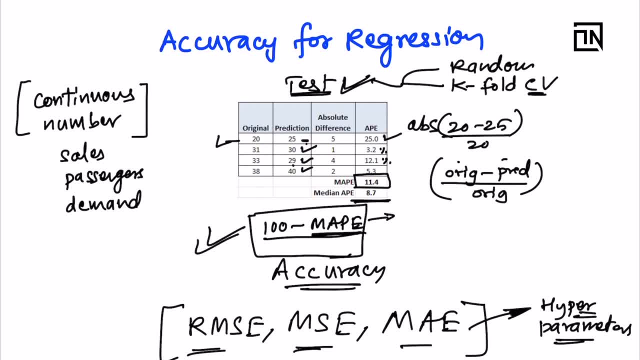 it. then accuracy is measured using 100 minus mape to explain to the client easily. all right, so do not use these in your answer. try to use hundred minus mape to explain to the client easily. 100 minus mape has your answer when you are giving it for the regression use cases. 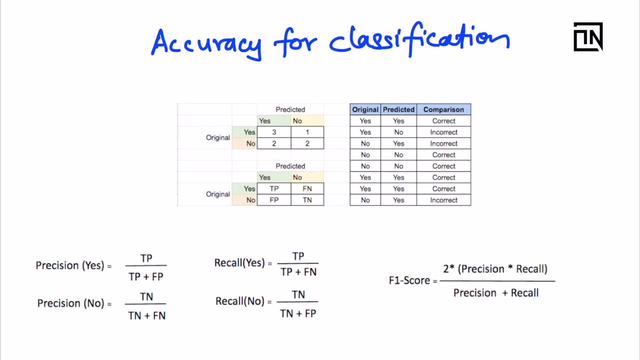 for classification. we know that classification is something when you predict a class and what kind of answers you are giving using a classification model. you are giving the answers like whether this loan should be approved or not, whether this transaction is fraudulent transaction or not. so this yes or no answer could be all the 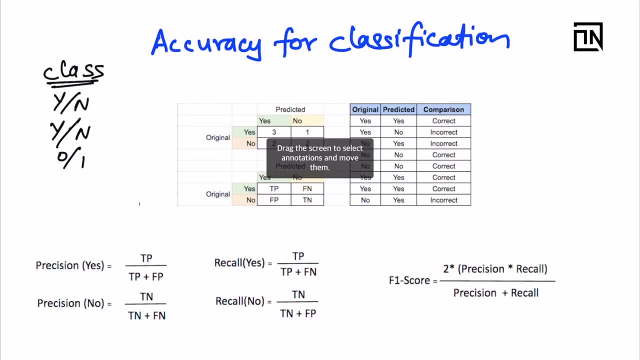 same. so, for example, if you are changing very much of class format or for example they have moved any class, set animals or maybe they have moved it, so a no old and active variety shape. so b1 also goes with this function, and 0, this very null, means centralised, �viol means 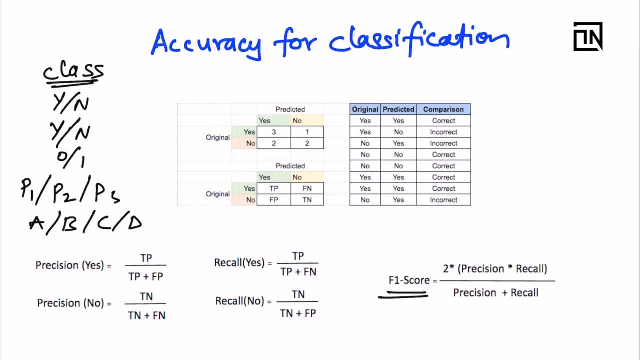 centralised spody, which meansuros. so all these things are constructed using this method. so, for example, we can try to use the formula: so you are saying that today you set theavian thumb issue and day thingi also number three model, which is mean the whole willジ record from 0-1 of z or 1 or 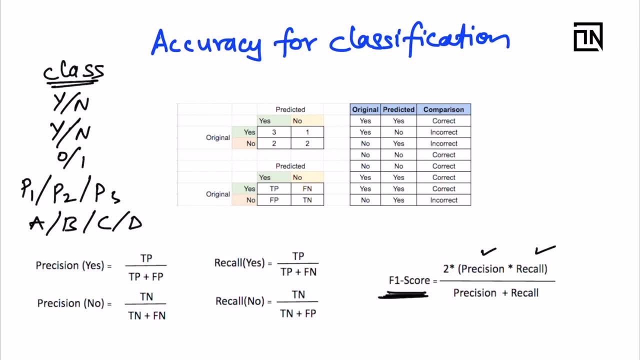 based on something which we call as a confusion matrix. So this which we, which I have created over here, is known as a confusion matrix. A lot of people will agree with the name: it's highly confusing, so so. so that's why the name. but actually it is derived from psychology. the kind of responses which 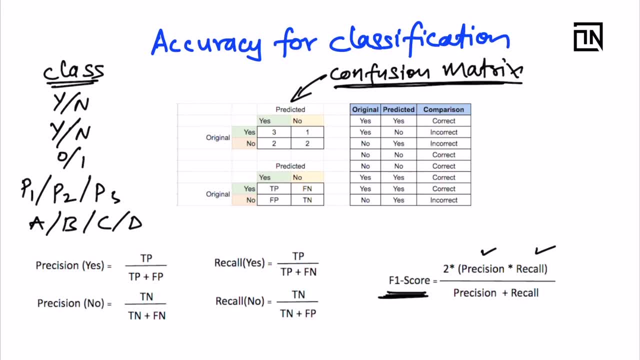 are standard versus the kind of responses given by a person or a test subject, and we are confusing these two metrics. so that is why it is known as confusion matrix. So this confusion matrix, what it tries to do is tries to see whether you have predicted the answer correctly or not. why are we doing? 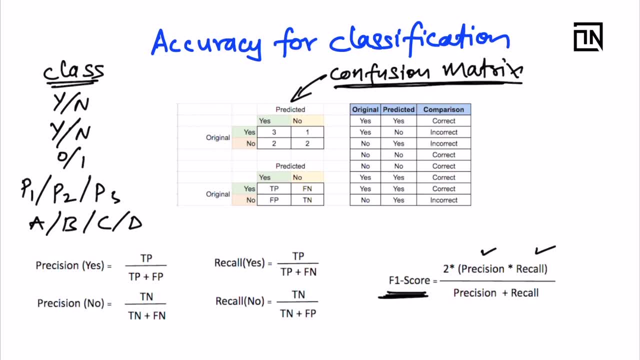 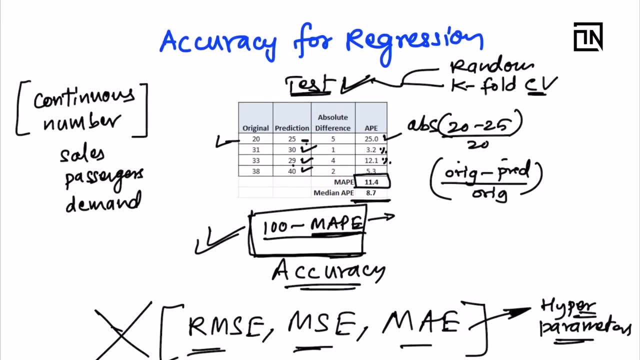 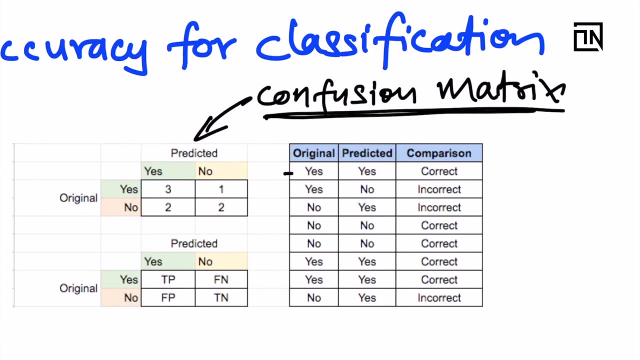 this: why are we not calculating the mean absolute percentage error, the absolute percentage error which we calculated here? this is something you cannot do on strings right, like for example here: the original value is yes and the predicted is yes. can you compute the absolute percentage error, the yes minus yes? it doesn't make sense. so when there 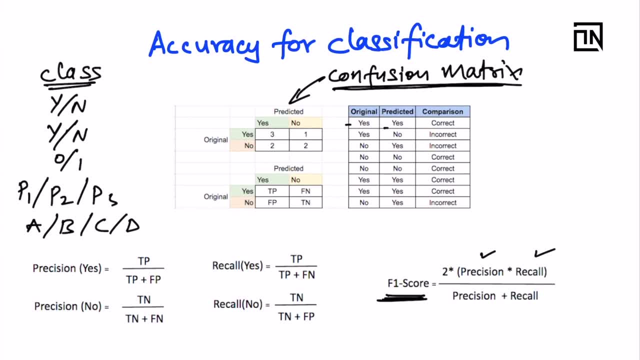 are strings specially. this is easy to understand. but even if you have numbers, mathematically you can compute the APE. but you should not, because that is wrong. you are doing classification. so in classification, when we cannot compute this, the difference between two strings or two classes, what we try to see, whether 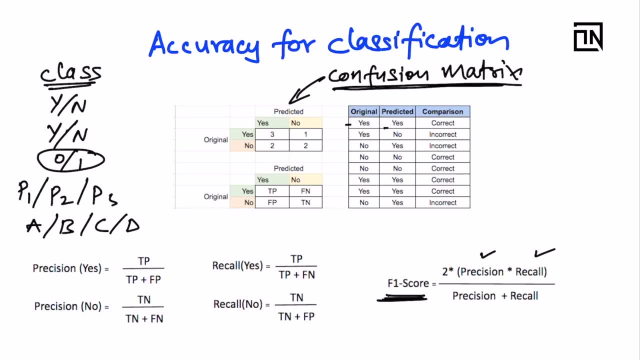 our model has correctly answered it or not. so originally it was yes and I have predicted it yes, so it is correct. yeah, this is my correct prediction. originally predicted as the. originally the value was yes and I have predicted as no, so this is incorrect. so this is the wrong answer. so I can do this. I can check how. 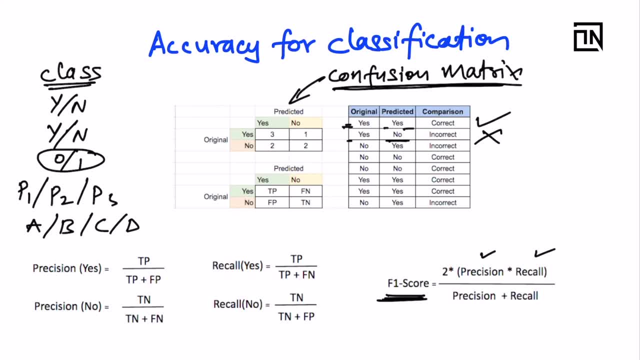 many correct answers I have given and how many incorrect answers I have given, and this is also one of the common mistakes. people simply take the diagonal element like yes, predicted as yes, so three values and no, predicted as no, two values. so people will calculate the accuracy of 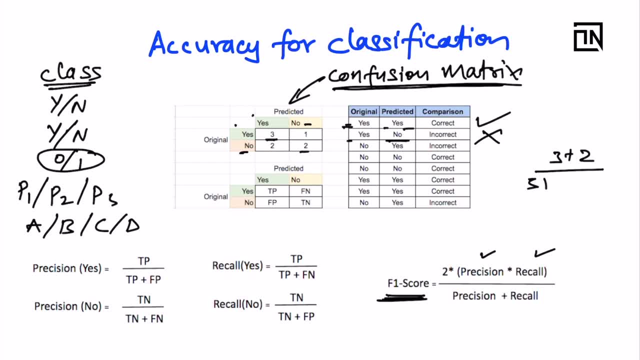 this model as 3 plus 2 divided by 3 plus 2 plus 2 plus 1, so all the cases which were correctly predicted plus all the other cases. so this is also known as the overall accuracy. so this is also known as the overall accuracy. 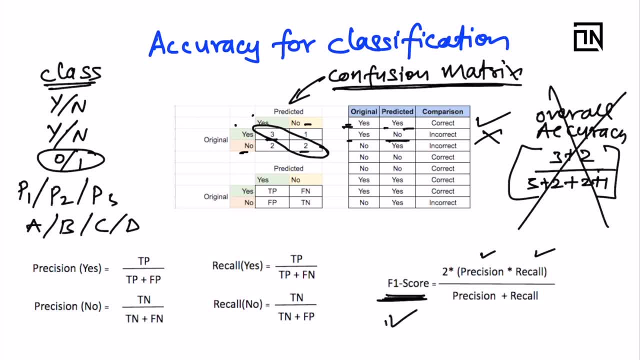 and this is not used in the industry. what we use is f1 score because overall accuracy disregards the bias of the data. like you can, you can simply say all, all answers as the majority class and still be- uh, still still have a high accurate model because of this flaw that it will simply take the 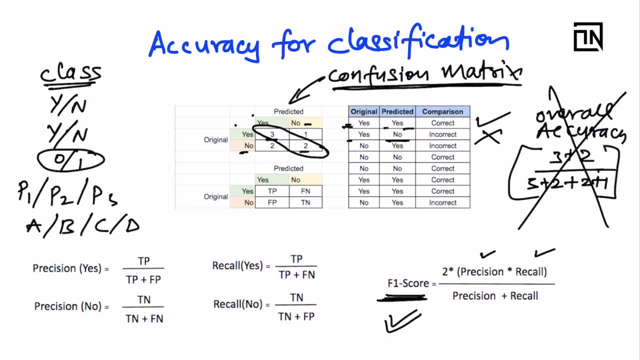 majority numbers as correct and divide by total numbers: okay, so we really care about how both the classes are correct. so we measure how precise the prediction is for yes class as well as no class, and we also measure how the recall of yes class and no class is individually, and then we combine. 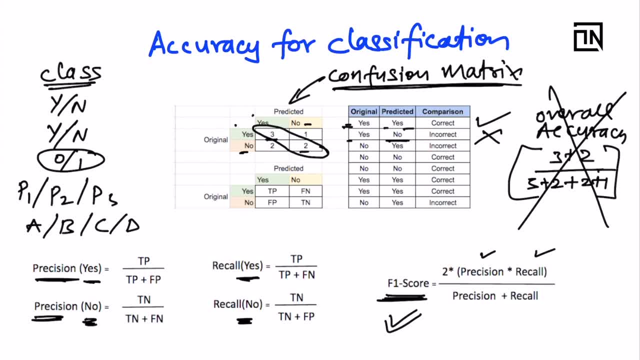 the precision and the recall value together and formulate an f1 score. so f1 score is calculated for yes class as well as for no class, all right, and this becomes the final answer. so f1 score really tells us like, uh, what is the predictive power of this classification model like? if the f1 score is 0.8, then out of out of. 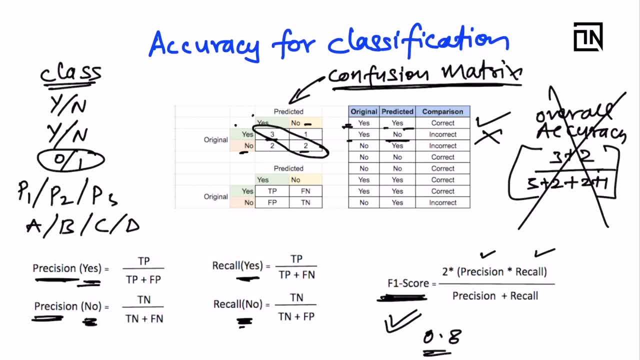 100 predictions, 80 predictions would be correct, which will comprise of yes cases also and no cases also, all right, so f1 score is the preferred metric, and overall accuracy is something which you should not use while deploying the model, because it may sometimes give you a very rosy picture, but you 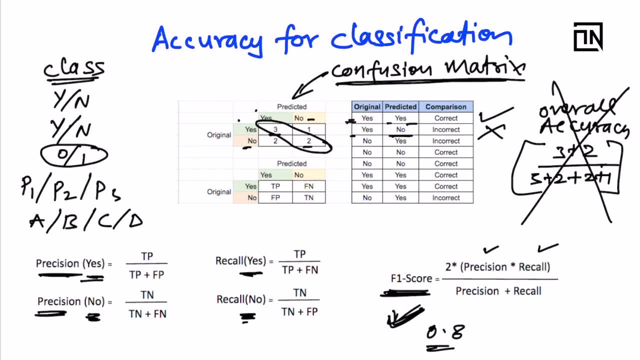 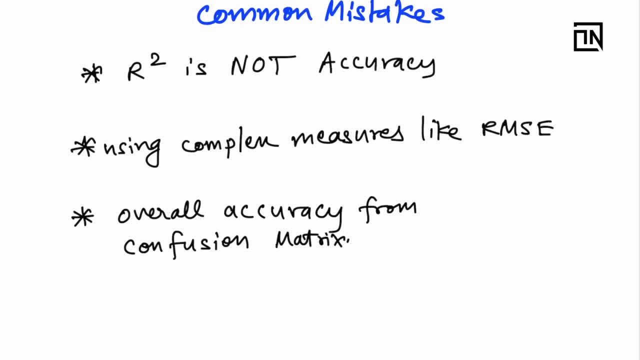 may, ah, find out later. you go and look at your evidence ALRIGHT. now let's talk about some of the common mistakes which is made by young data scientists. a lot of people i have seen use r square as a metric for accuracy, so r square is not accuracy. 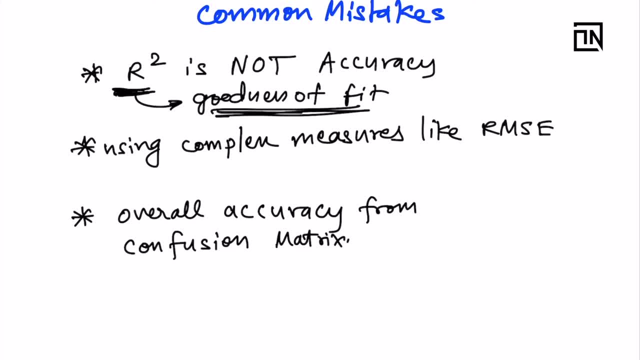 r square just represents, goodness of it, variance. your model has explained It is not the accuracy metric. Yes, the accuracy metric is interlinked with R-squared. If your model has a high R-squared value, then you will get a good testing accuracy as well. But it is not always correct. Your model could be. 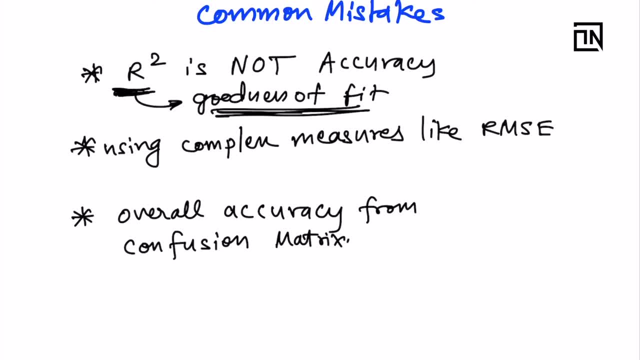 an overfit model as well, where the R-squared value will be really high. But when you test the model on the testing data, the testing accuracy may come very low because of the overfitting. So R-squared is not a metric to be reported as the accuracy of the model. 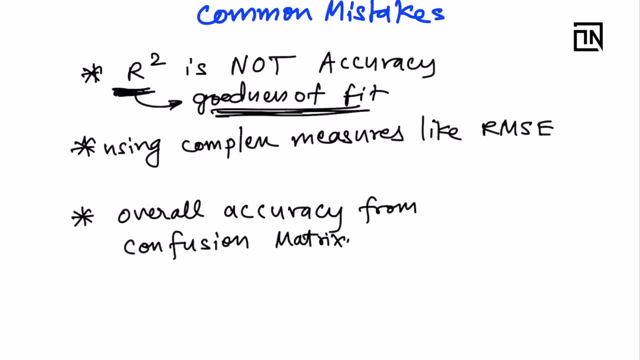 It may lead to some unexpected results. So you will say my model is 90% accurate by looking at the R-squared. But when the client is comparing the predictions with the actual value, they will say that your model is 90% accurate, but why the values are coming so far away? 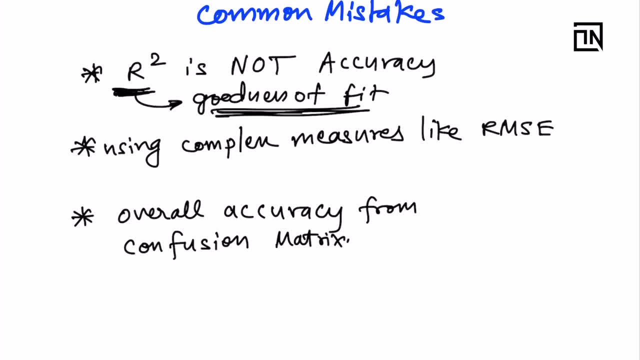 So testing accuracy needs to be employed to set up a realistic expectation with the client. And if you start talking in terms of complex measures like RMSE, so it is good for your evaluation. As a data scientist, you understand them easily, But sometimes your client is not from statistical. 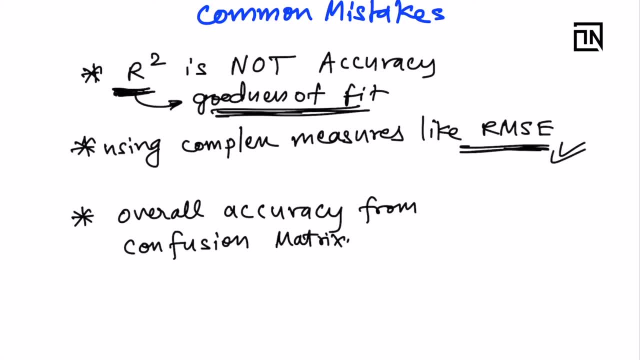 background and they will not be able to talk in these terms, So you will have to go down to the terminology which is easier and universal to understand, like percentage difference. So this is the original, this is the prediction, and how much percentage difference is there? 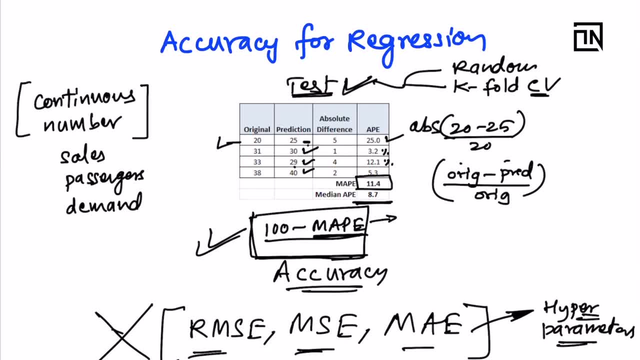 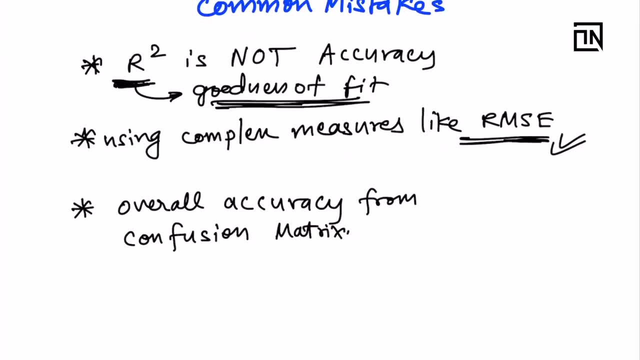 And, as we saw, the metric which we use is mean absolute percentage. So this is the difference between the M&A and the FNN score, And the FNN score is the overall accuracy and the percentage error in these scenarios. Similarly, in the classification case, using the overall accuracy,